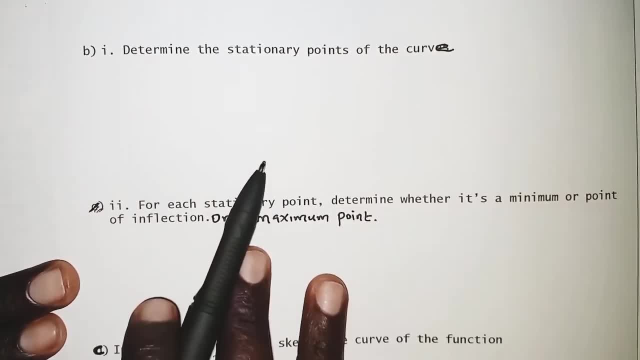 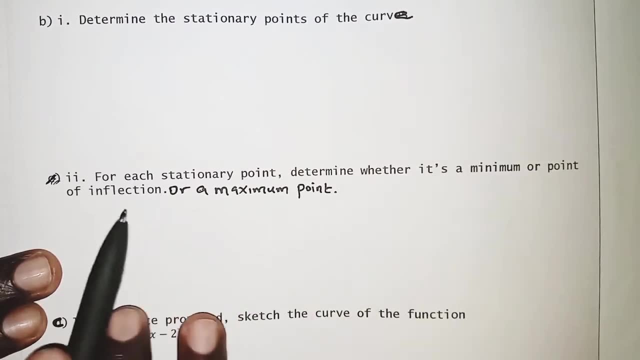 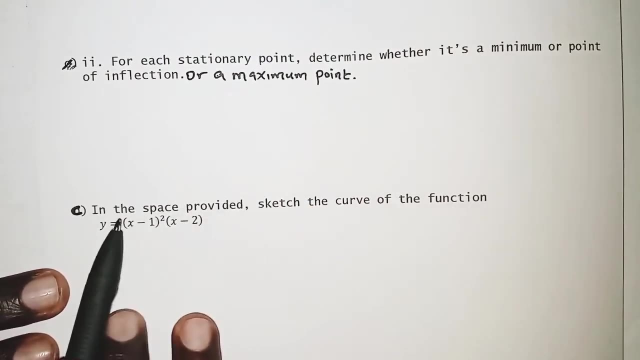 the stationary points of the curve. then b roman 2, for each stationary point, determine whether it's a minimum or point of inflection or a maximum point. Then, lastly, in the space provided sketch, the curve of the function y is equal to x-1. 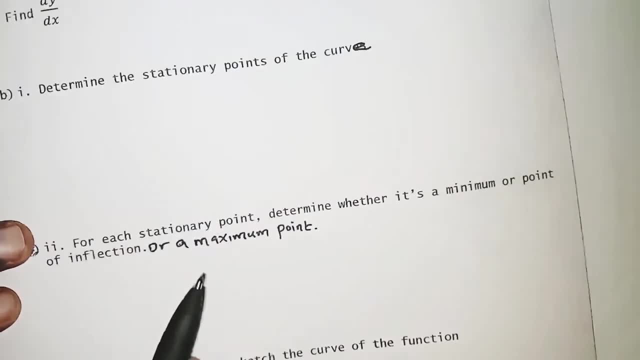 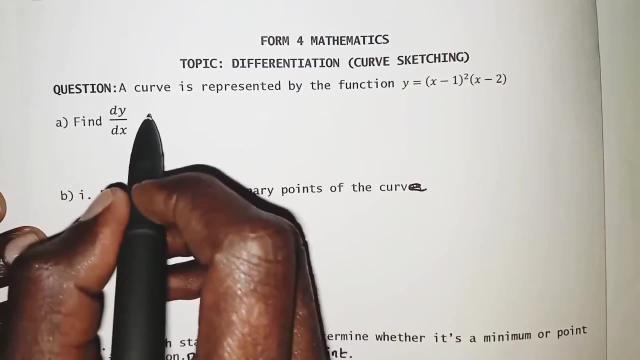 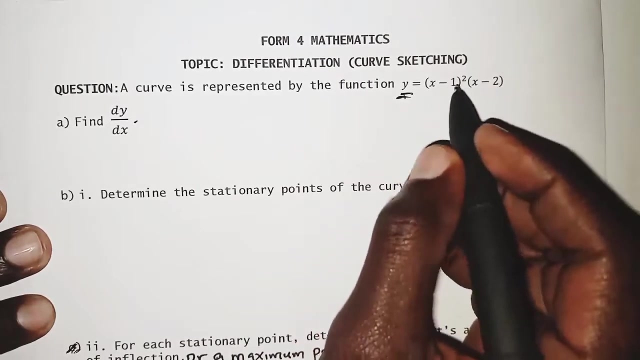 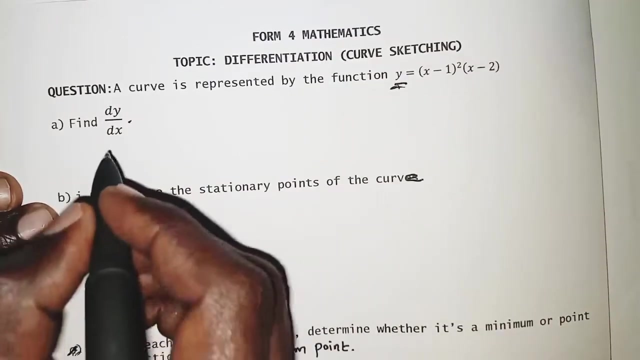 squared into x-2. So here. so for part a, we are required to get the derivative of this function here. but before we do that, the first thing we'll be required to do is to expand. so we'll have: y is equal to so. 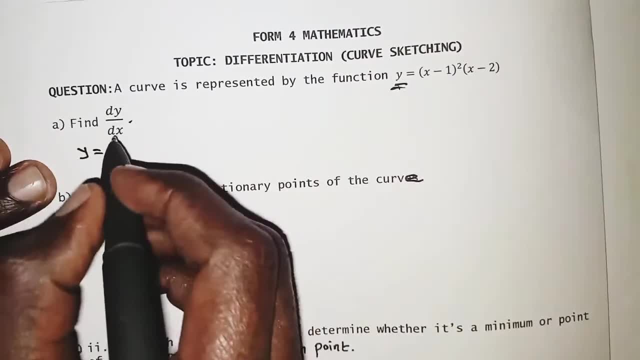 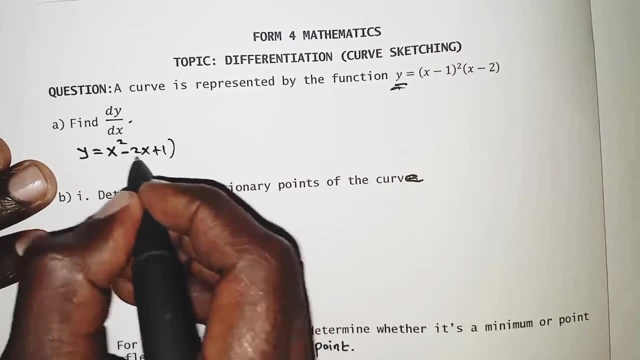 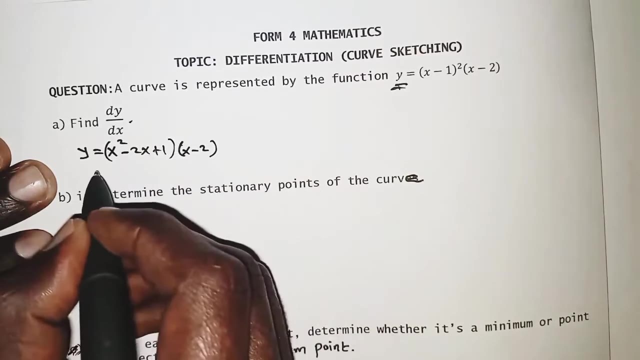 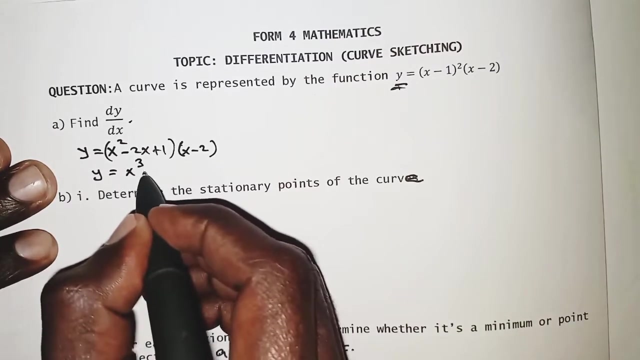 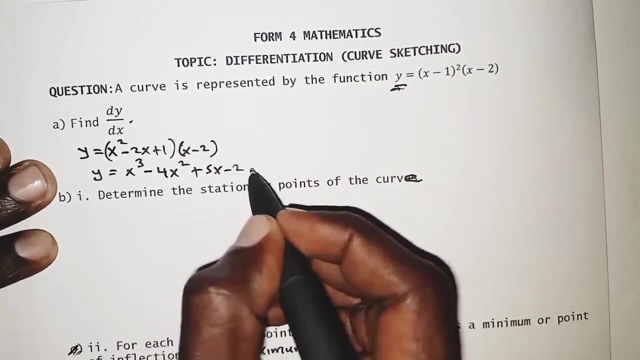 for the quadratic part x-1 squared, we'll have that expanded as x squared minus 2x plus 1, and then we multiply by the other part, x-2.. So this, when expanded, should give us x cubed minus 4x squared plus 5x minus 2, and therefore 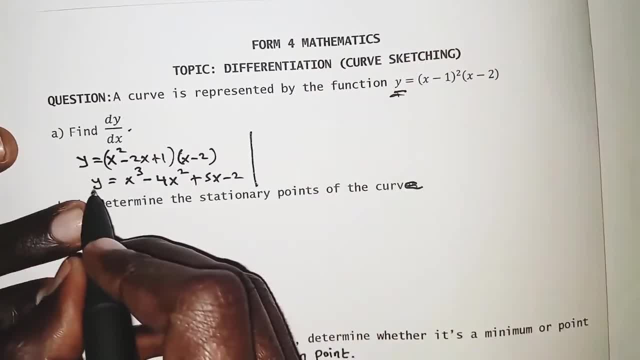 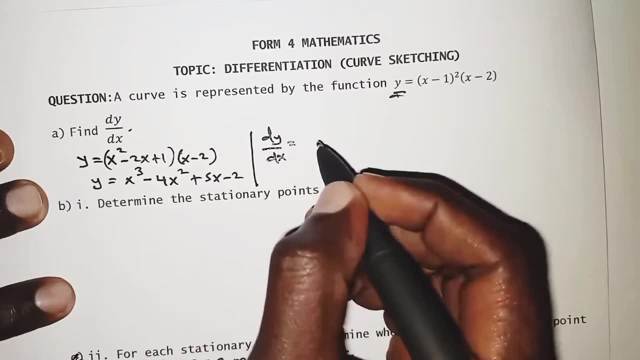 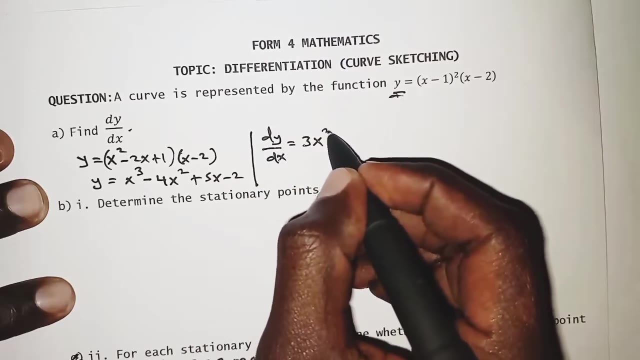 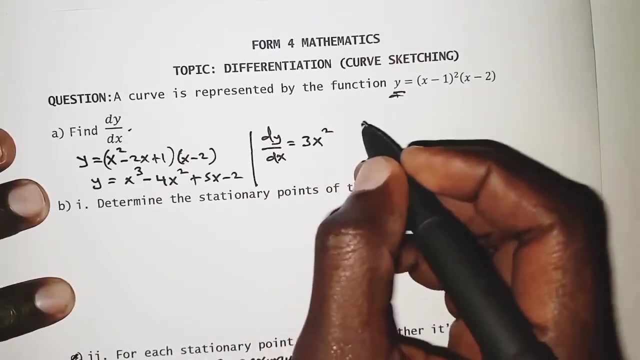 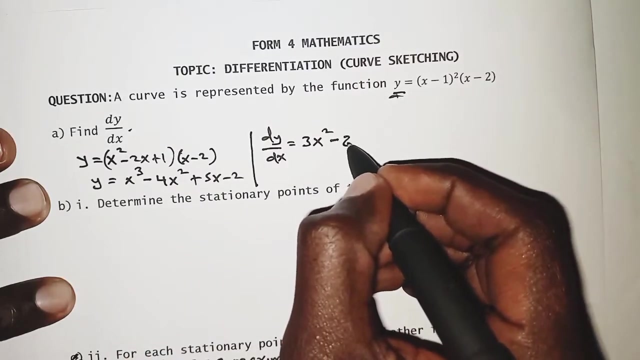 from there we can now get the derivative of y with respect to x, that is, dy over dx. So this should be given as 3x squared. So we have 3x and then the power reduces by one minus 2, by 4, that should give us 8x, and 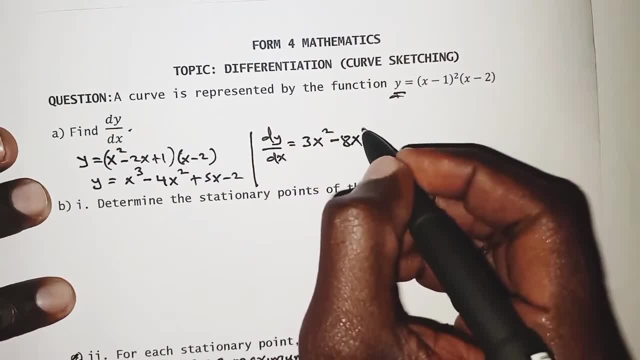 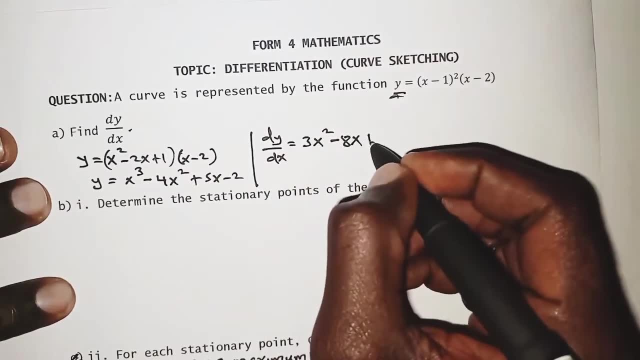 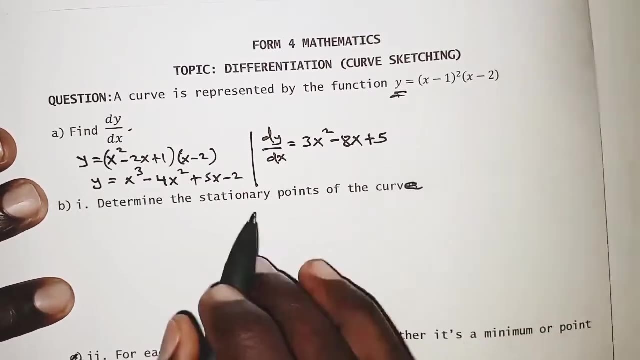 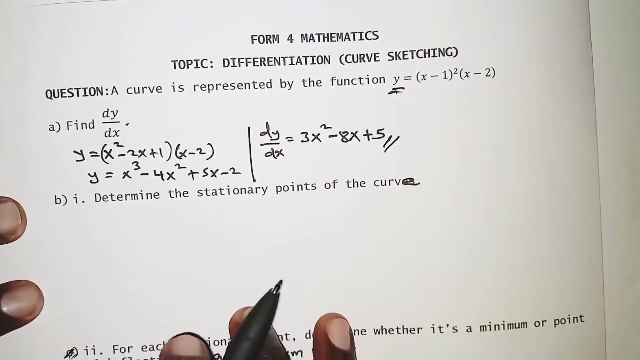 then the power reduces by one. so we have 2 minus 1, so x power 1,, which is just x, and then plus 5x, when differentiated becomes 5.. So this is the derivative of y with respect to x. For part b: determine the stationary points of the curve. 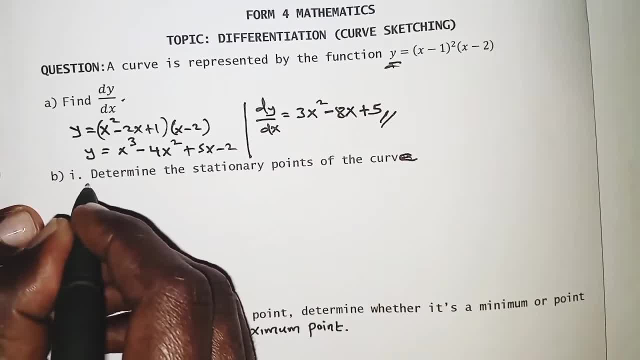 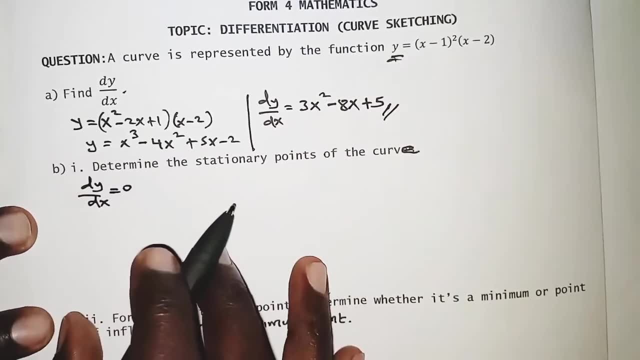 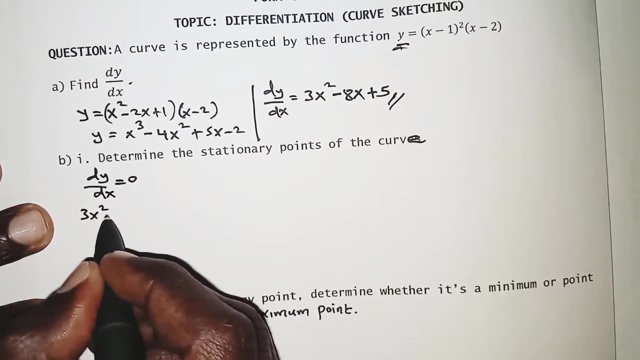 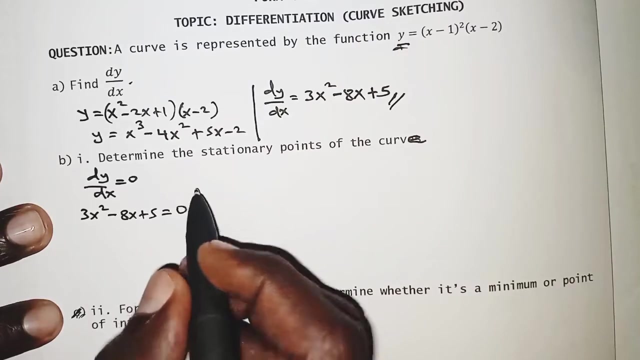 So at stationary points we know that the derivative of y is is 0, that is, dy over dx is 0. So already you have gotten dy over dx to be 3x squared minus 8x plus 5.. So that is 0. 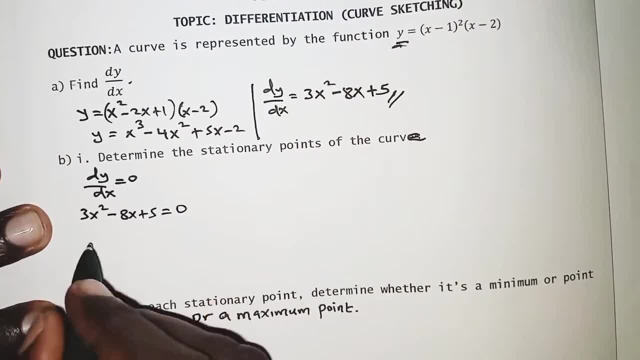 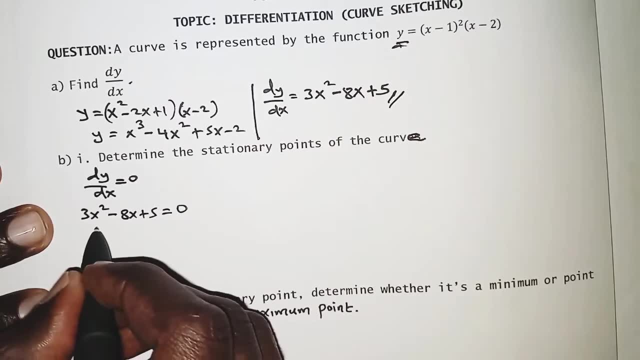 When this is factorized on the left hand side, in order to solve for x we are going to have, so use factor method. So the point is 0. The product of two factors, rather, is 15.. So we have 5 by 3, giving us 15.. 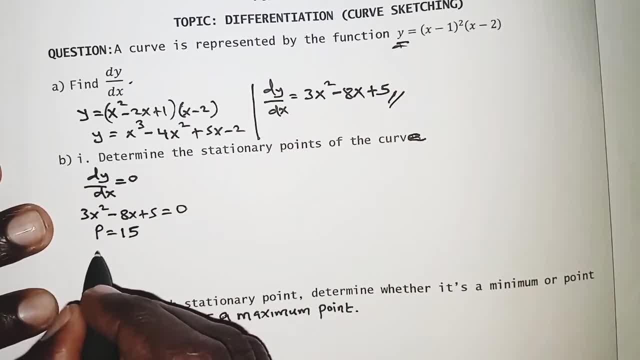 So the product of the two factors we are looking for and then the sum should be negative 8.. So the factors are negative 3 and negative 5. So multiply them, We get positive 15 and then we get negative 8.. 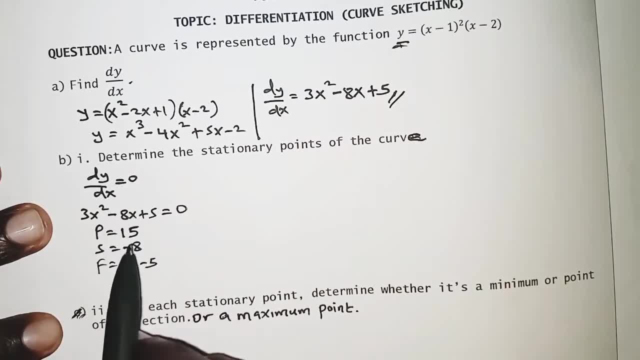 So we are going to replace negative 8x with negative 3 and negative 5x respectively, So that we are going to have the equation written as 3x squared minus 3x minus 5x. that in place of negative 8x. 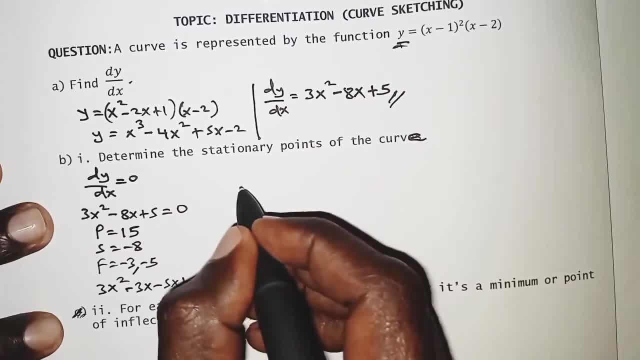 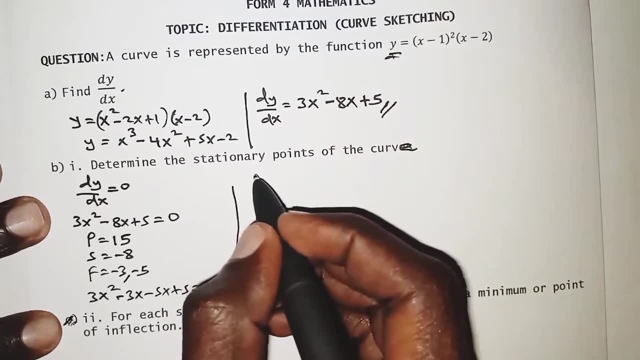 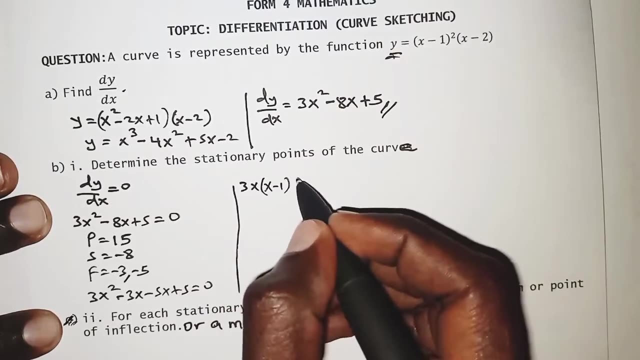 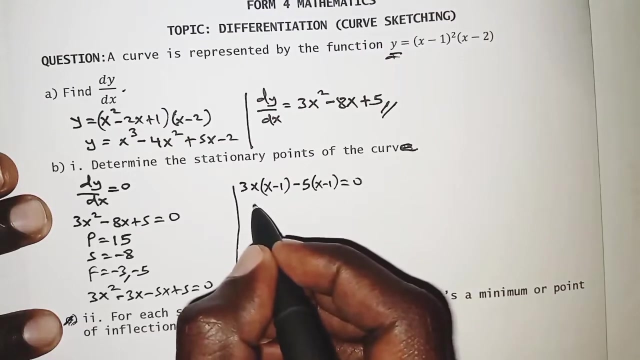 Plus 5 is equal to 0.. From there we can now factorize the left hand side so that we have 3x into x minus 1 minus 5 into x minus 1 is equal to 0. So this becomes x minus 1 into 3x squared minus 3x squared minus 3x squared minus 3x. 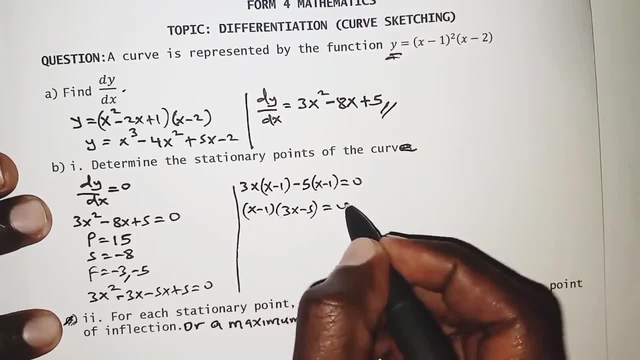 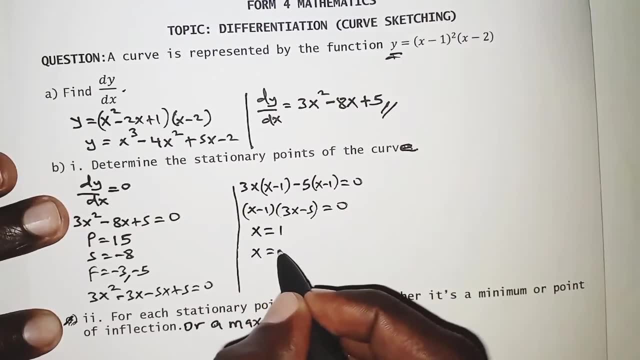 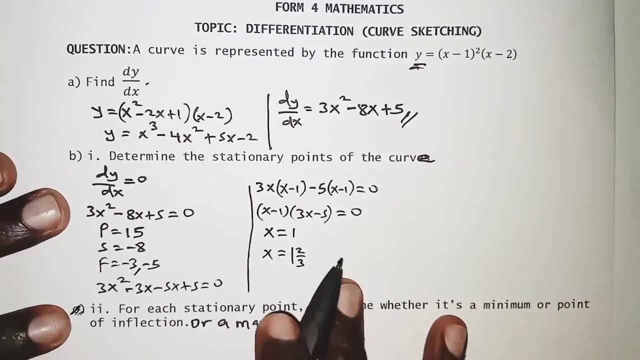 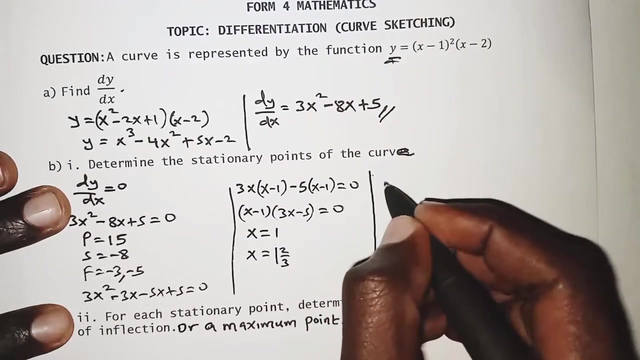 squared, x minus 5 is 0.. So from here we can get x to be 1 and x is 1 and 2 thirds. So from the values of x we can now get the y coordinates, So if x is equal to 1.. 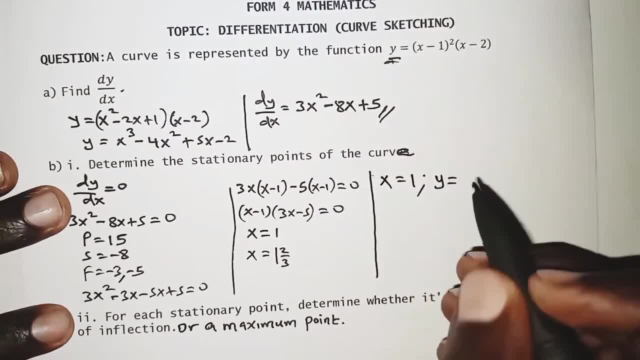 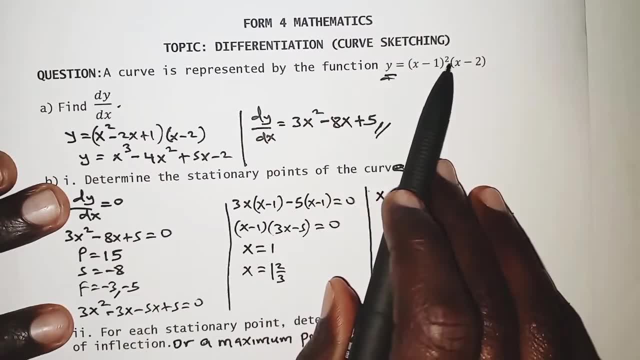 Then y is equal to 1.. Then y is equal to 1.. Then y becomes so: this we are going to obtain by simply substituting back in the original function. So y is x minus 1 squared into x minus 2.. 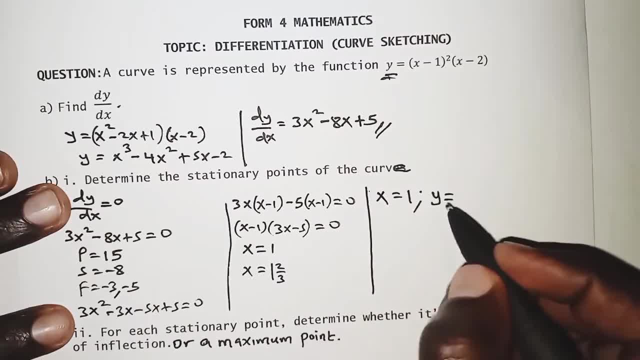 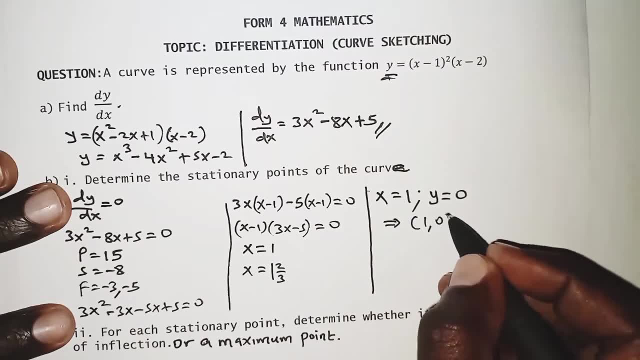 So when x is 1, we realize that y becomes 0. So this gives us the point 1 comma 0. So 1, 0 is 1 of the stationary coordinates. So we can now multiply both sides So y becomes. so this we are going to obtain by simply substituting back in the original. 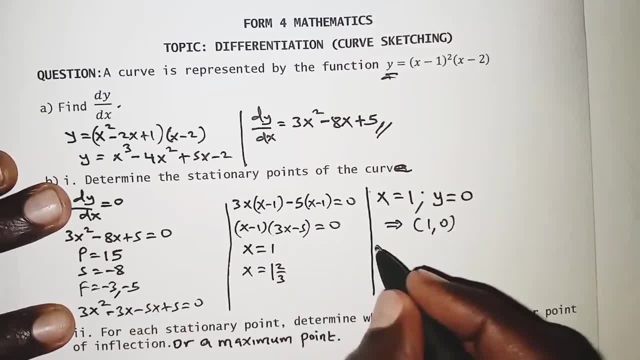 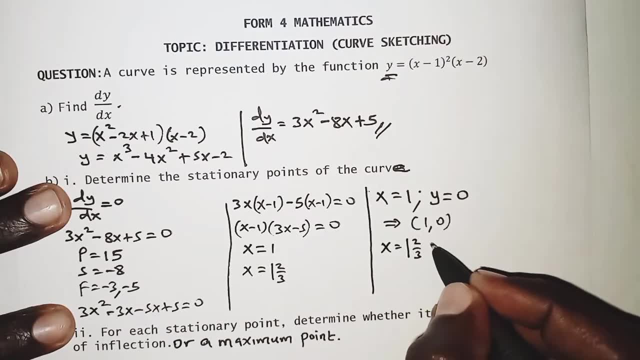 one of the stationary points. Next, when x is 1 and 2 over 3,, y becomes. so when you substitute back, what you are simply going to have is negative 4 over 27, so that the point becomes 1 and 2 over. 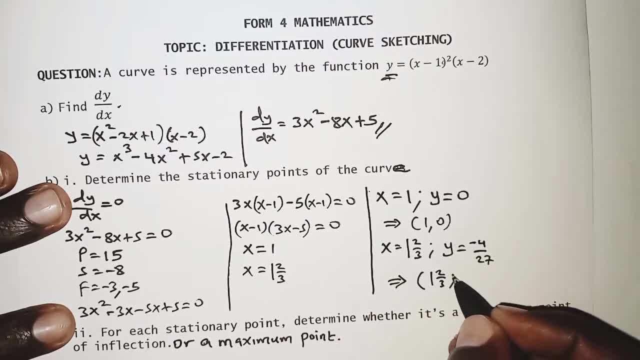 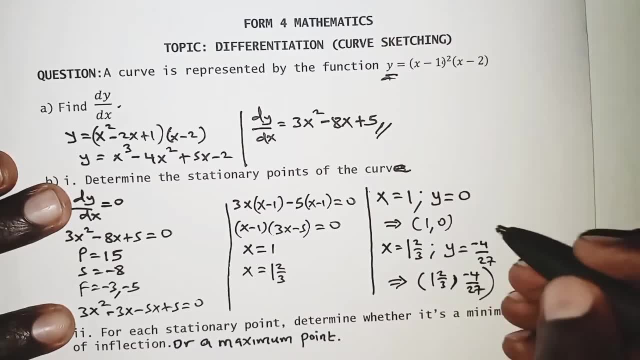 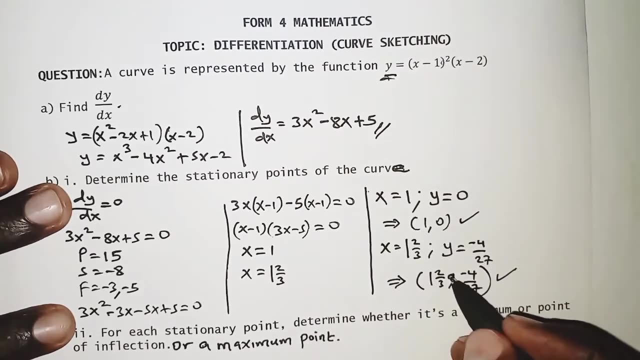 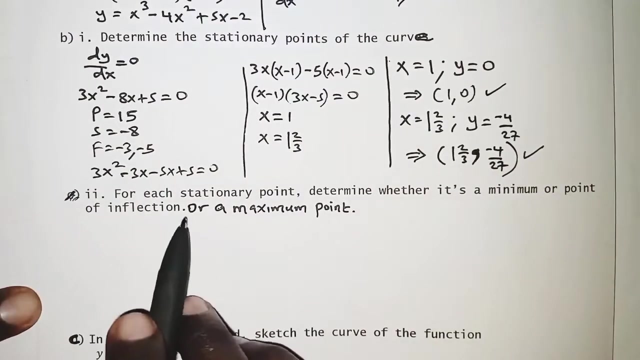 3. sorry, sorry, comma negative 4 over 27.. So these two points are the stationary points. So sorry, this is a comma. Okay. so for the next part, for each stationary point, determine whether it's a matrix or a模. 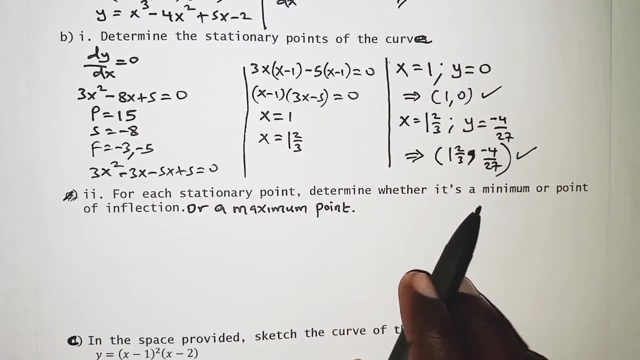 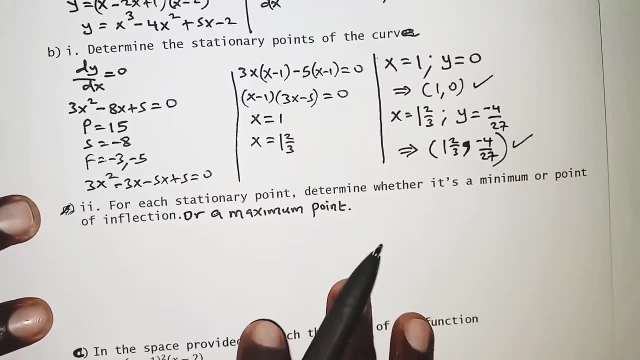 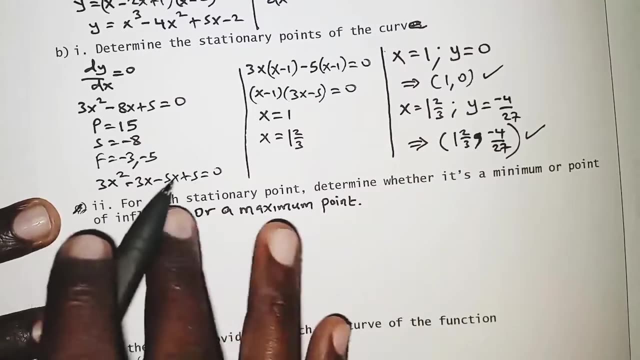 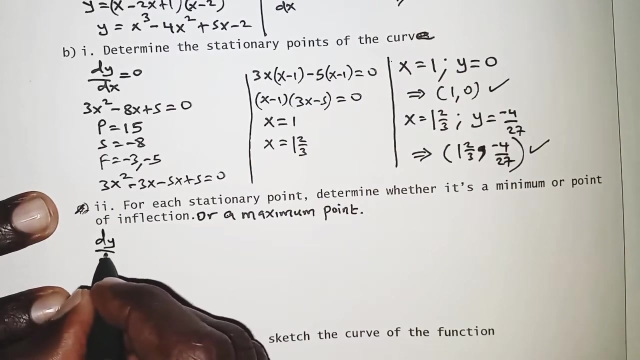 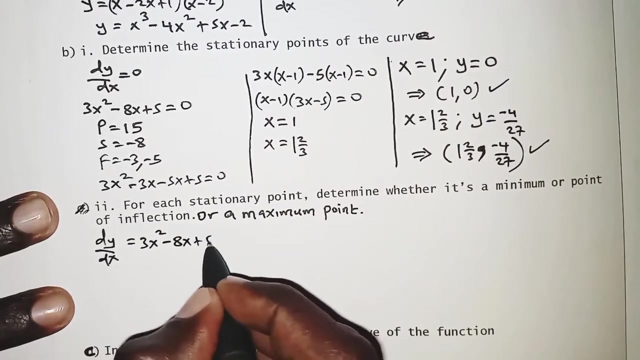 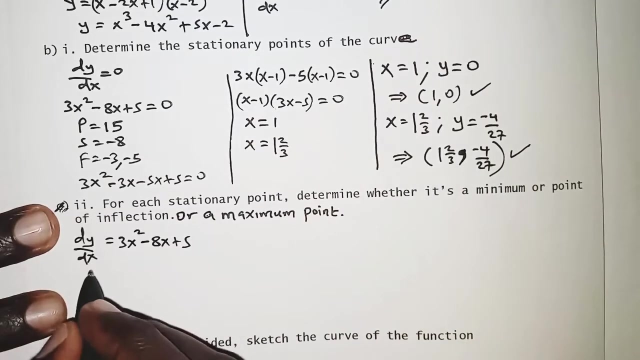 or maximum, or a point of inflection. so here we are going to use the second derivative to do the test. so the first derivative, which was dy over dx, we had gotten to be 3x squared minus 8x plus 5. that is, from up here now differentiating. 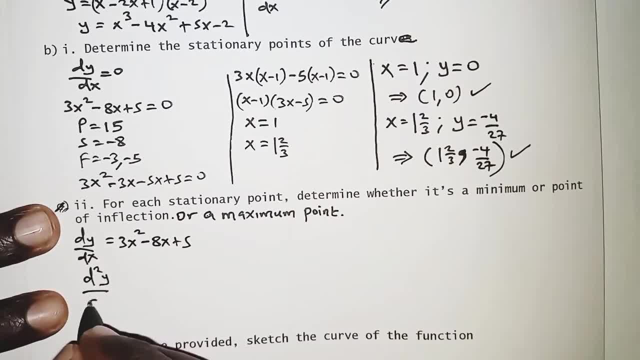 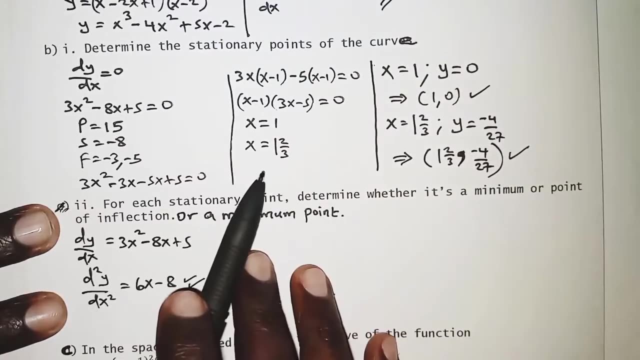 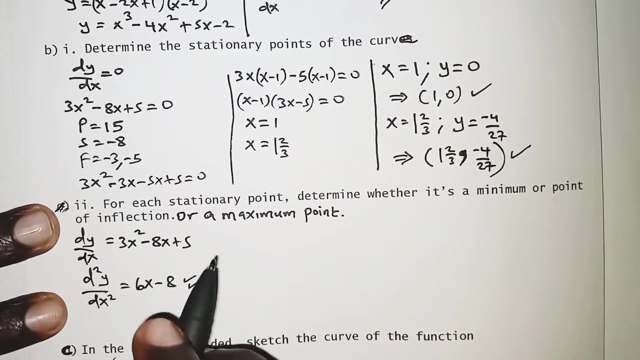 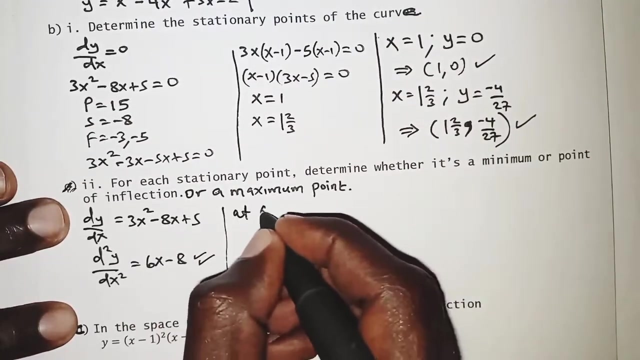 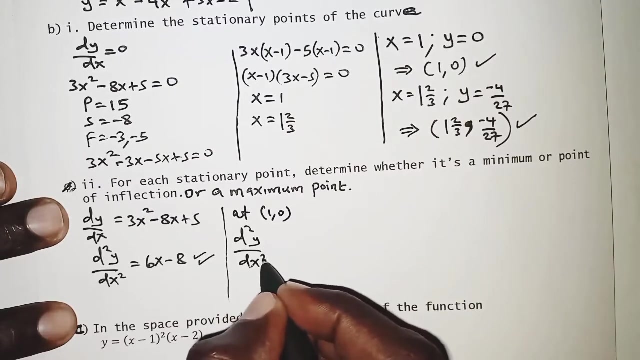 a second time. we are simply going to have 6x minus 8. so using the second derivative we can tell whether the points above a maximum, a minimum point or a point of inflection. so at point 1: 0 the second derivative simply becomes. so we substitute the value of X. 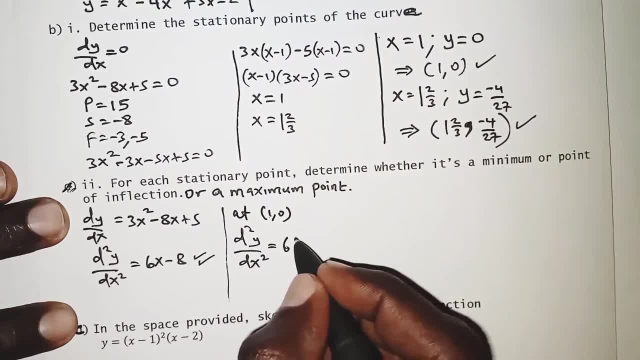 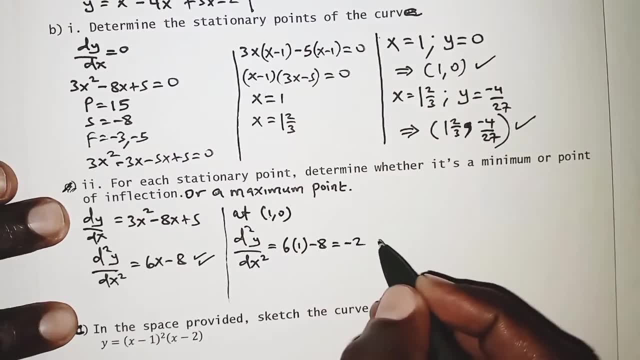 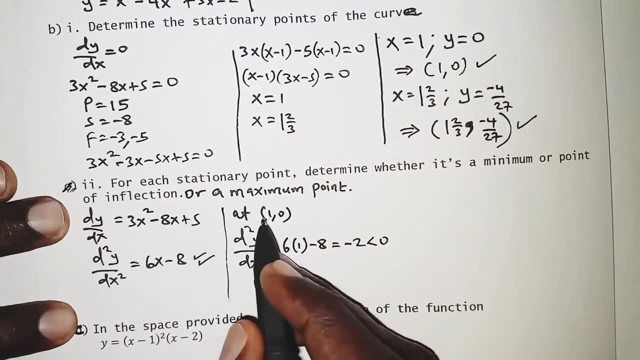 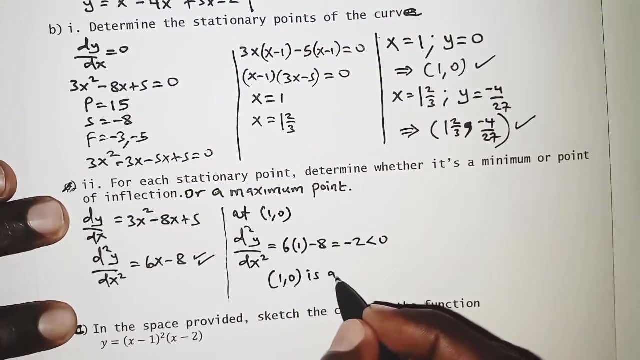 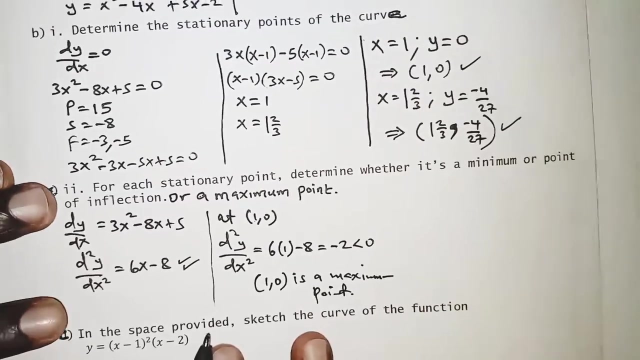 of which in this case is 1. so we have 6 into 1 minus eight and that is negative two. so negative two is less than zero. so if the second derivative is less than zero, then that point is a maximum point. so point 1- zero- is a maximum point. next we are going to test. 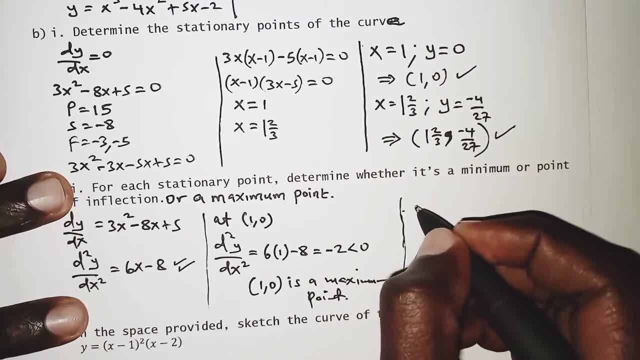 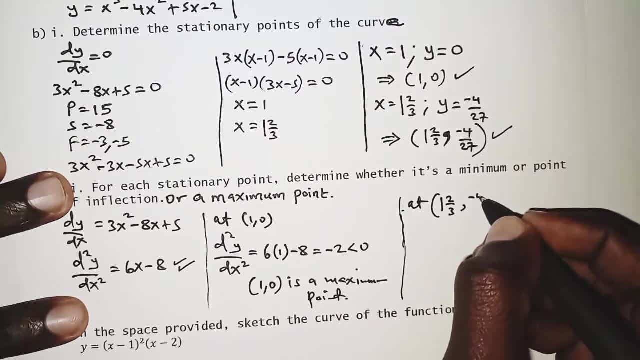 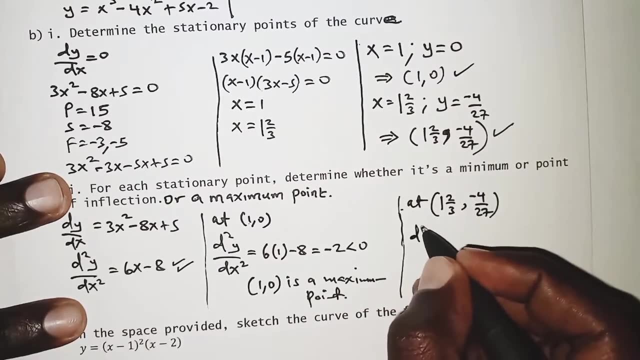 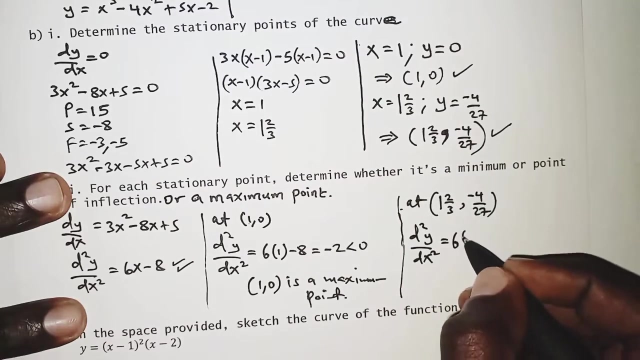 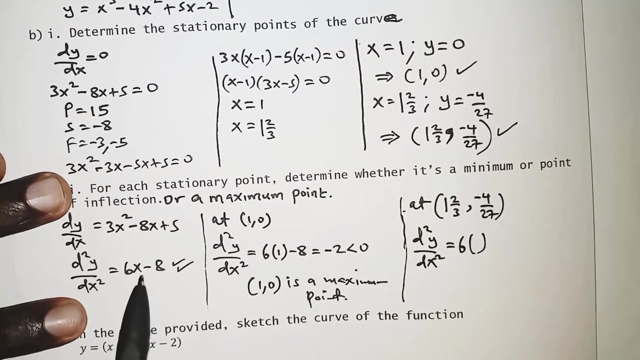 the nature of point 1 and 2 over 3 comma negative 4 over 27.. So the second derivative simply becomes 6 and then we substitute the value of x. Remember we are still applying this second derivative. so x for this particular case is 1 and 2 thirds. 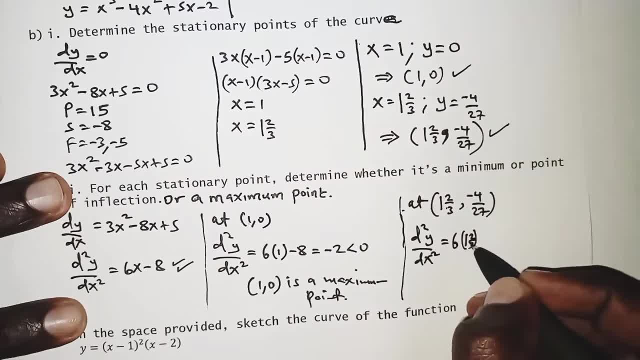 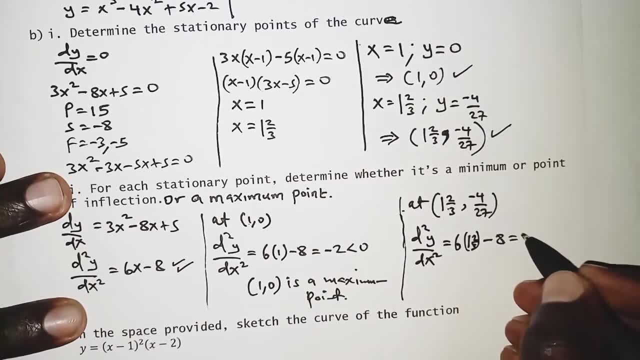 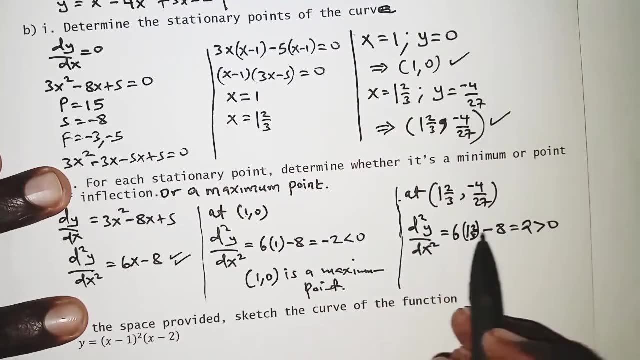 so 1 and 2 thirds minus 8, so this is going to be 2 and for this case 2 is greater than 0.. So if 2 is greater than 0, or in other words, if it is positive, then we substitute the value of x. 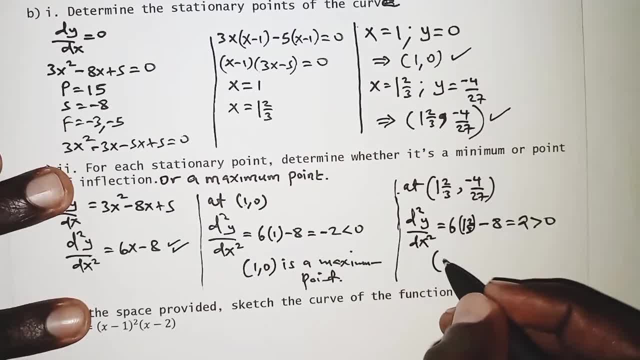 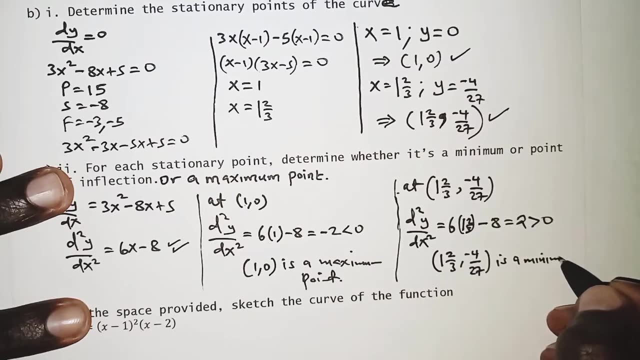 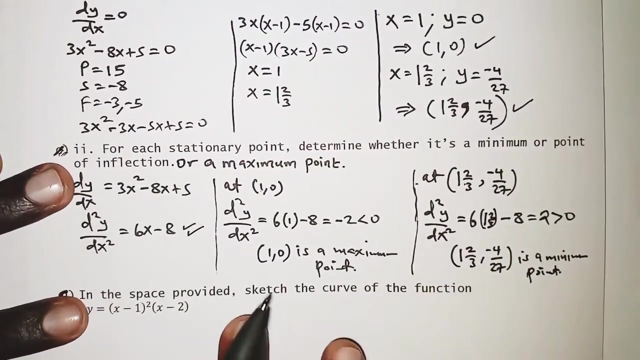 and we substitute the value of x, Then that particular point- like here we have 1 and 2 over 3 comma negative 4 over 27- is a minimum point, And thus we have determined the nature of the points. Suppose the second derivative was: 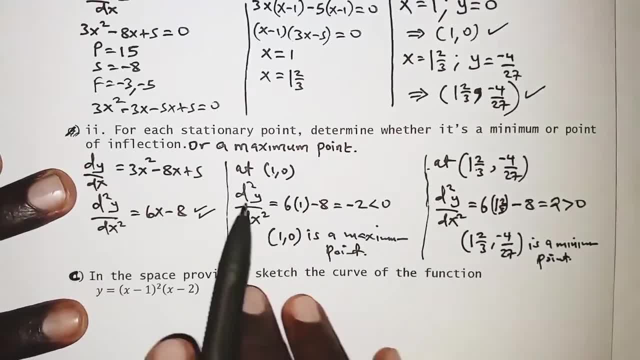 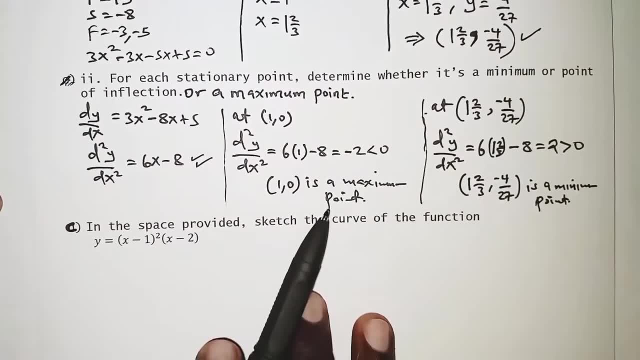 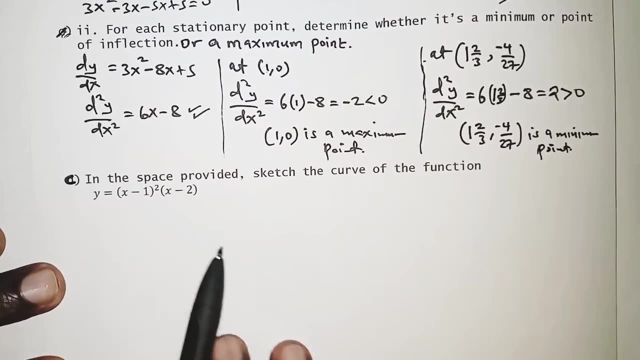 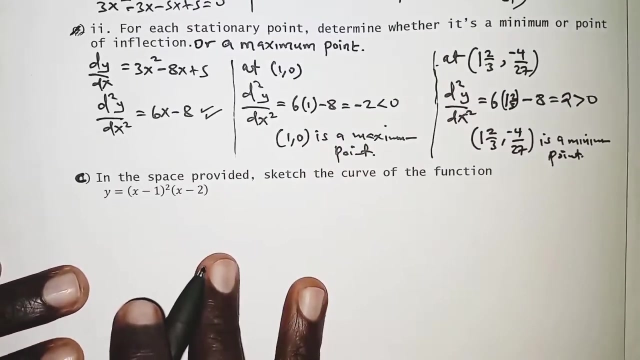 equal to 0, then the point would qualify to be a point of inflection. So next we move to the last part. In the space provided, sketch the curve of the function. So for us to get, or rather to sketch the curve, then what we need to know is that: 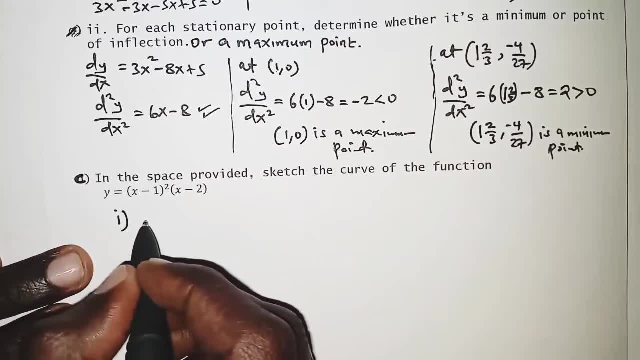 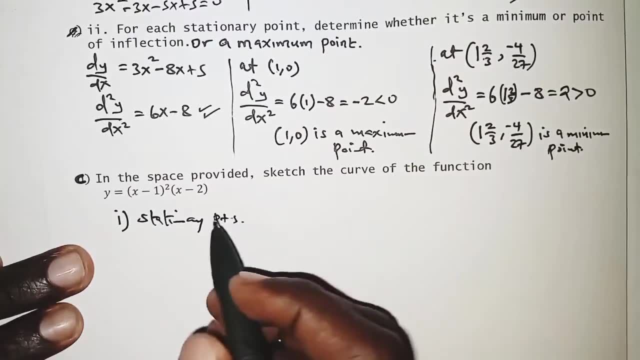 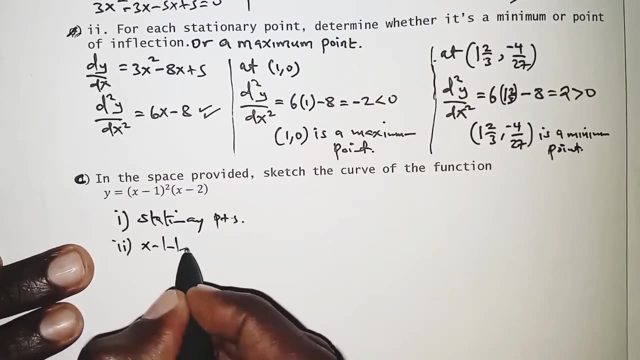 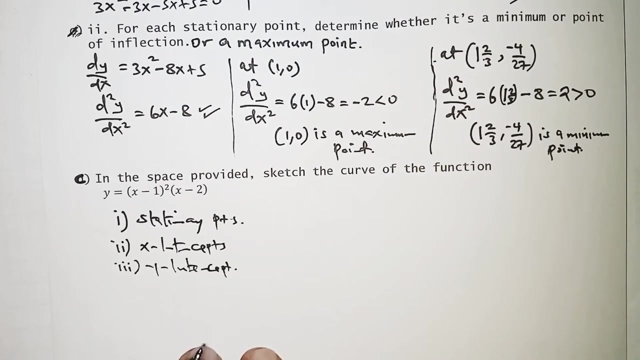 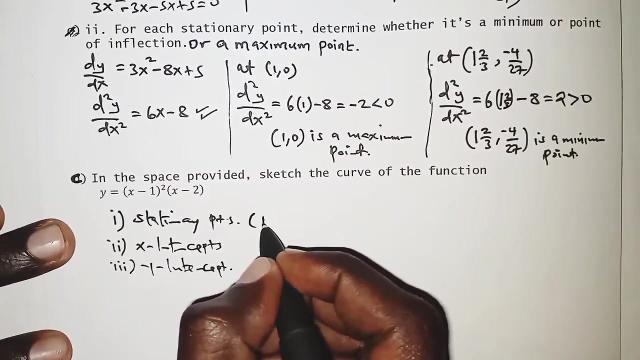 we need to know is number 1: stationary points, which are the turning points. We need to know x-intercepts and we also need to know the y-intercept. Those are four points, Three important components. So already we know the stationary points, which we got to be 1, 0 and 1 and 2. thirds: 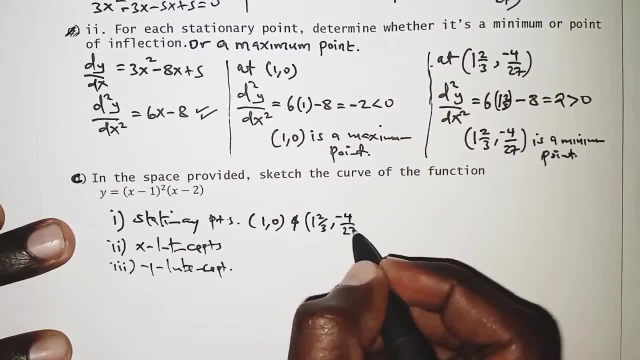 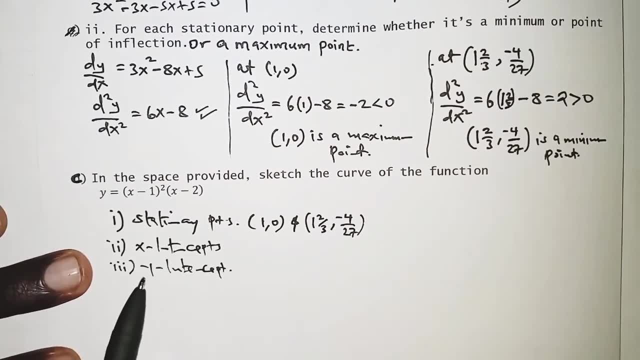 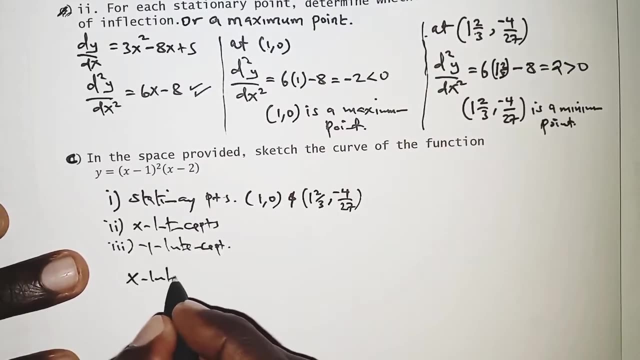 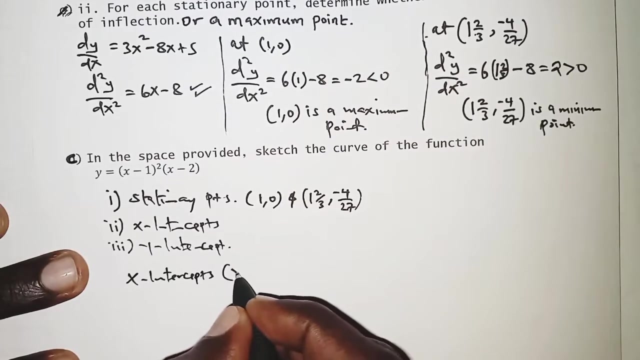 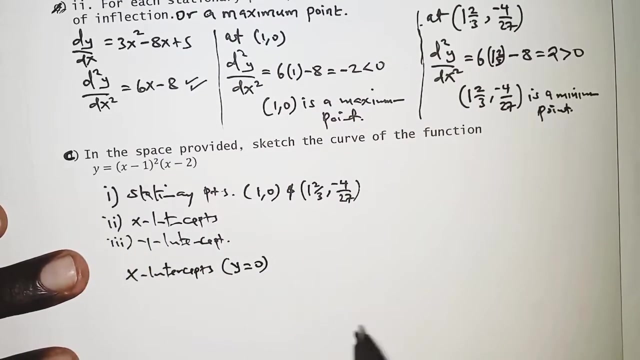 negative, 4 over 27. So we are yet to determine the x-intercepts and the y-intercepts. So at the x-intercepts we know that y is 0. So we substitute that in the function here. So we have: if y is 0. 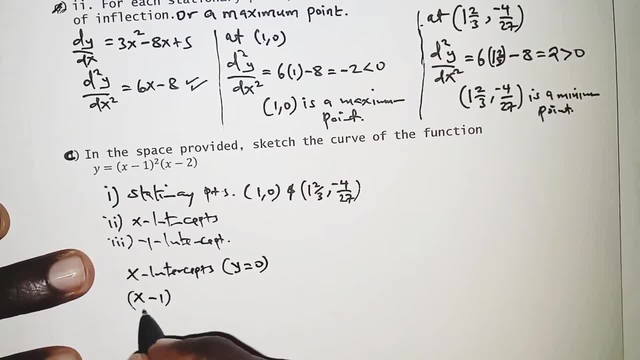 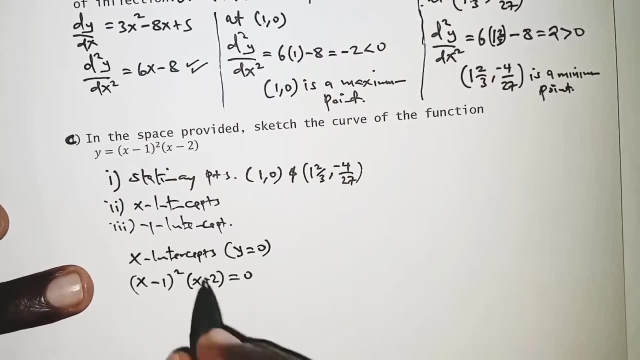 we will have x-1 squared into: x-2 is equal to y, which is 0.. So from here we can see that x-2 is equal to y, which is 0.. So from here we can see that x-2 is equal to y, which is 0.. 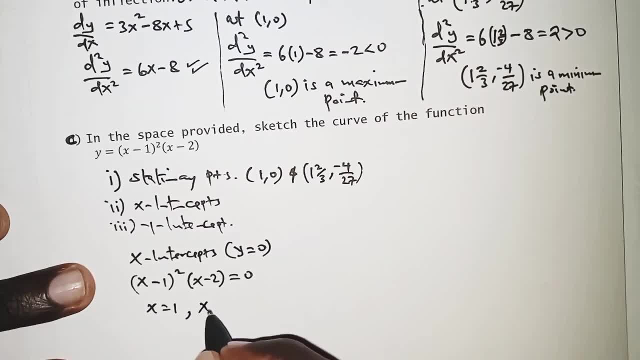 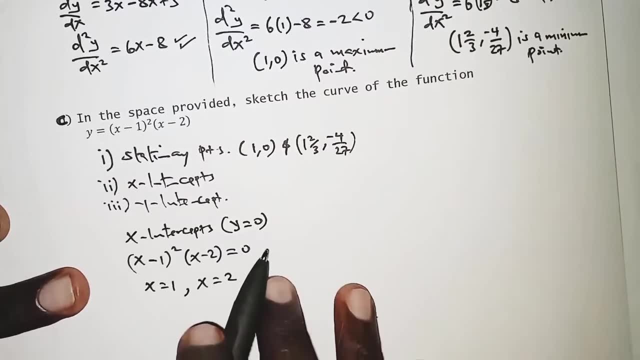 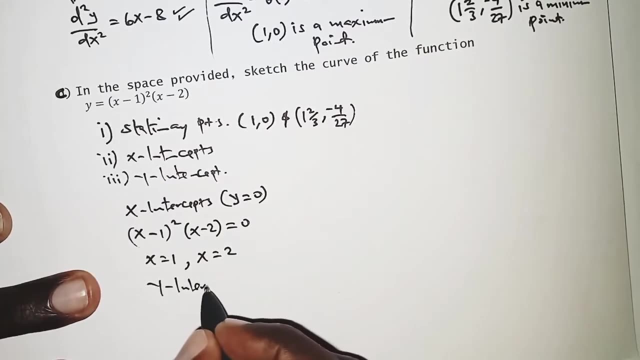 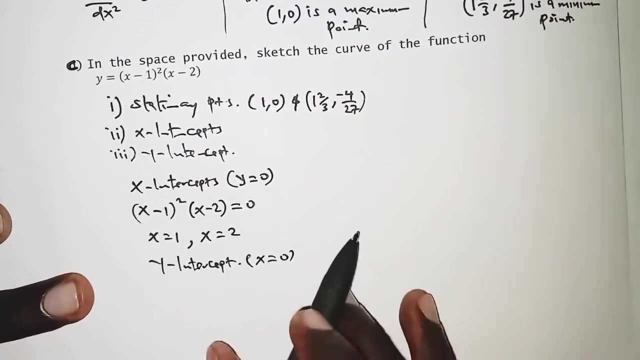 We can see that x is 1 and x is also 2.. So x is either 1 or x is 2.. and then we can also say for the y-intercept x is 0. So we substitute in the function there. 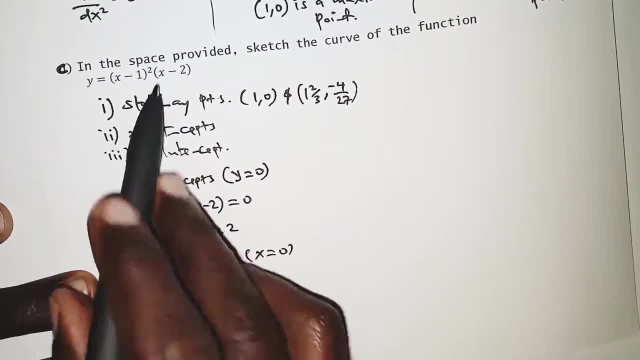 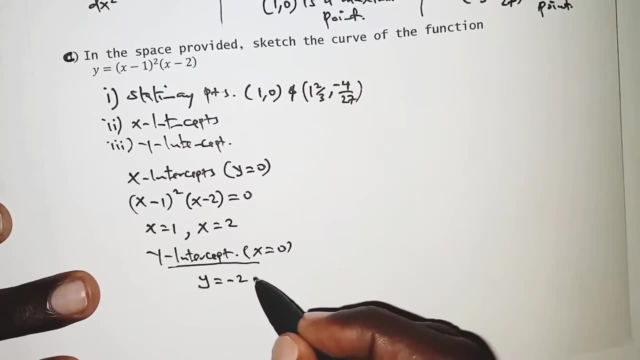 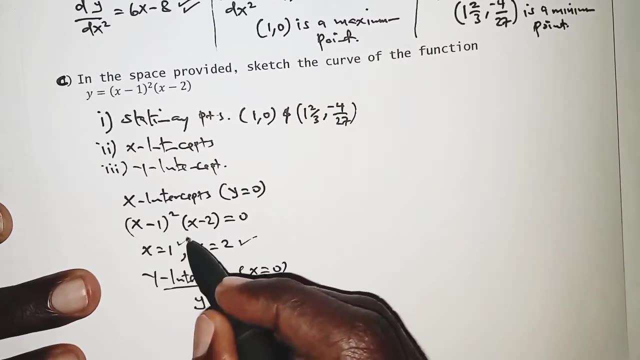 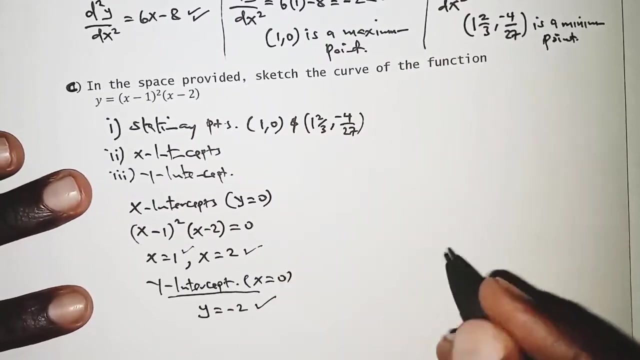 So that when we substitute x is 0, then we will get that y becomes negative 2. So the y-intercept is negative 2, the x-intercepts are 2 and 1. So with this we can now sketch, So in. 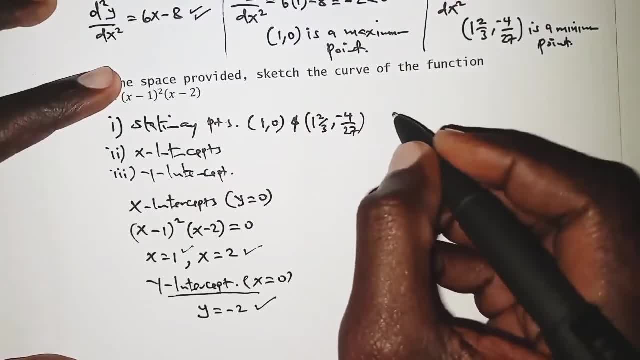 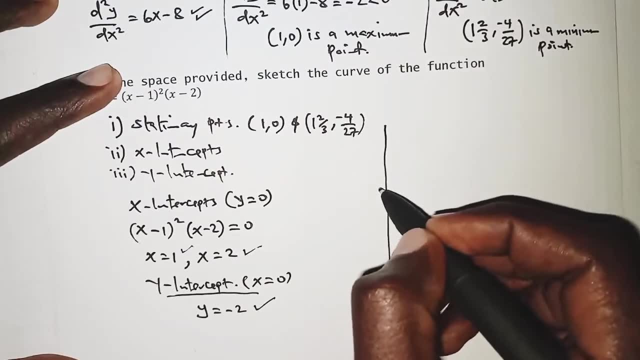 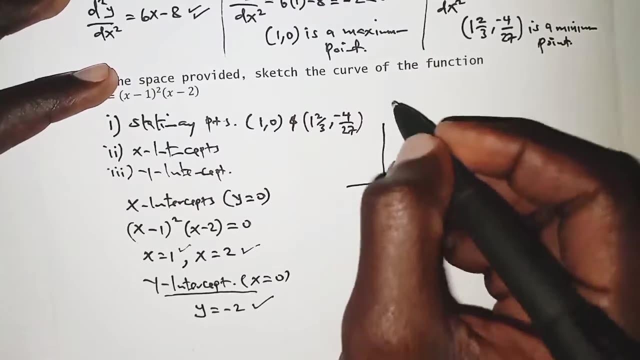 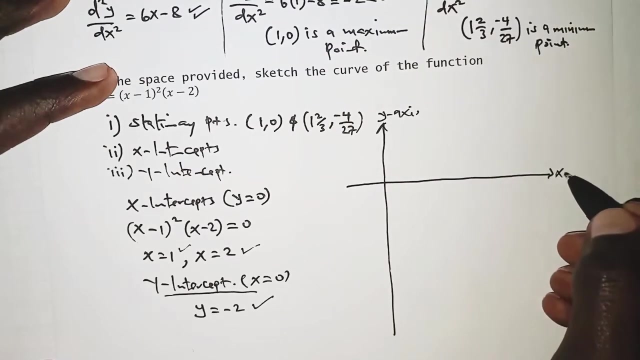 sketching. we can use straight lines, So make use of a ruler to draw straight lines. So this is the Cartesian plane. This is now y-axis, and then, right here, we have the x-axis. So we are going to locate the x-axis. So we are going to locate the x-axis. So we are going to locate. 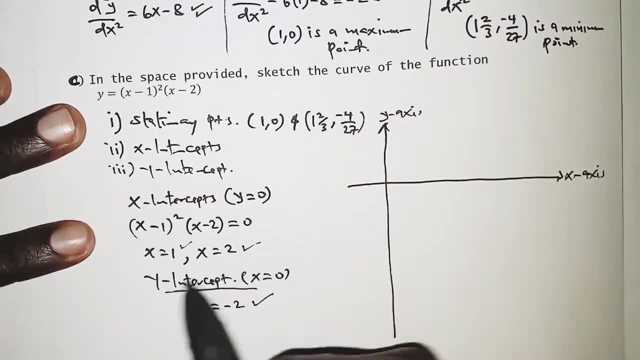 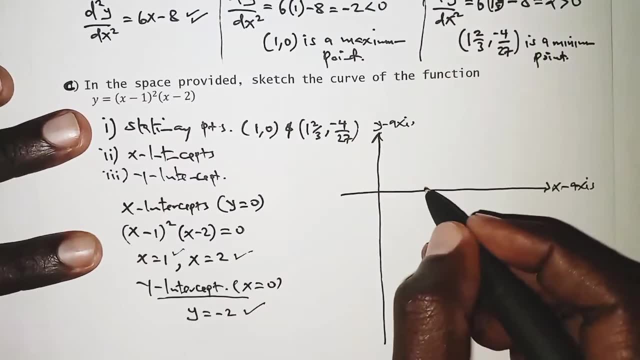 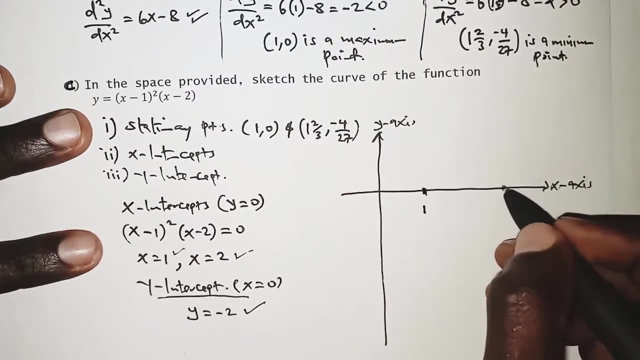 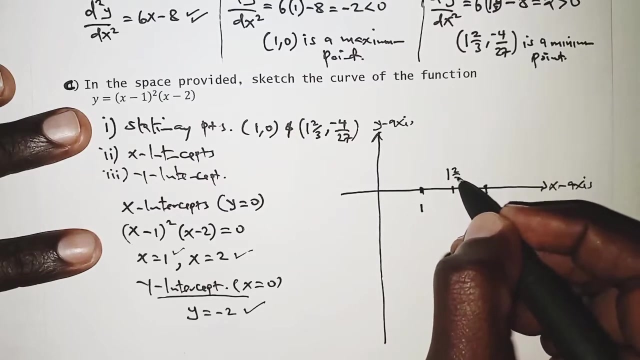 these points the estimate positions. So for us to locate 0.10 then we must be somewhere at 0.1. Then 0.1 and 2 over 3, somewhere between 1 and 2.. So we know it's somewhere here, 1 and 2 over 3.. And for negative, 4 over 27. we 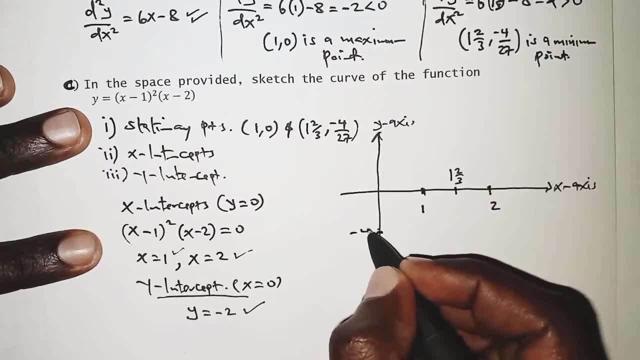 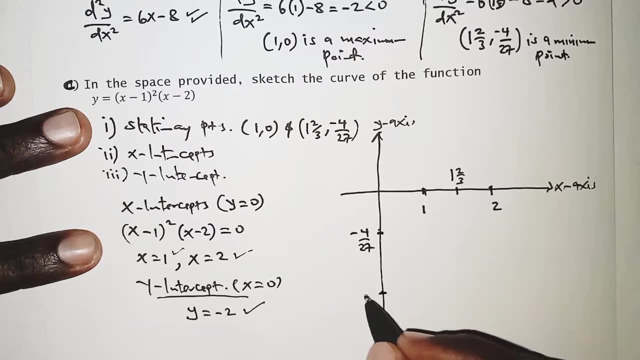 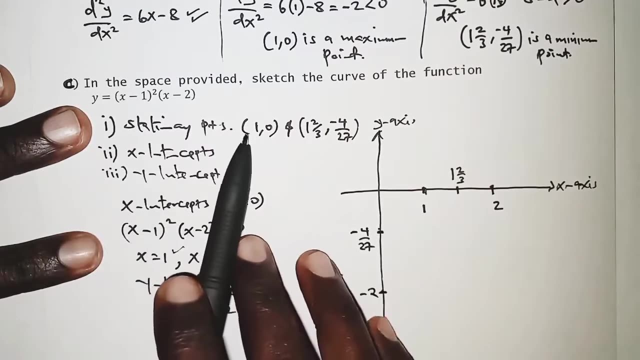 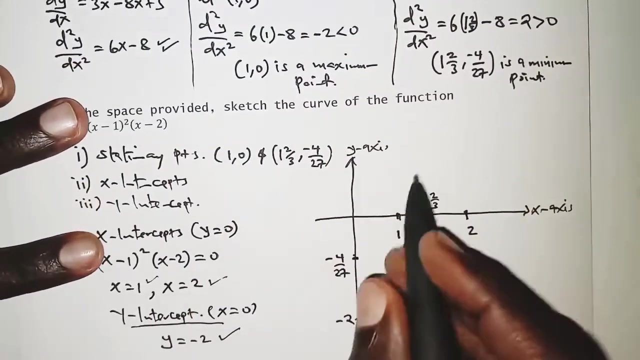 can have it somewhere here- negative 4 over 27. And then the y-intercept negative 2 we can have down there. So for the stationary points, or the turning points, we have 0.10 and 0.10 we had identified as a maximum point, So sorry. 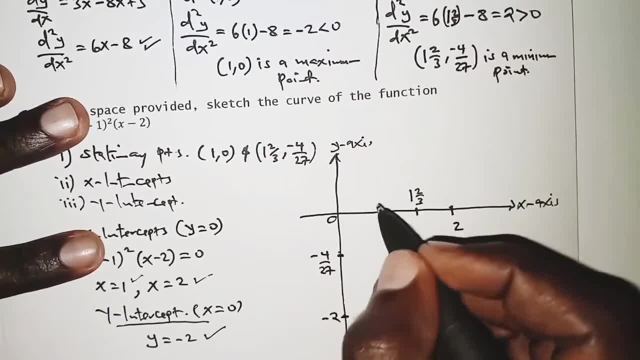 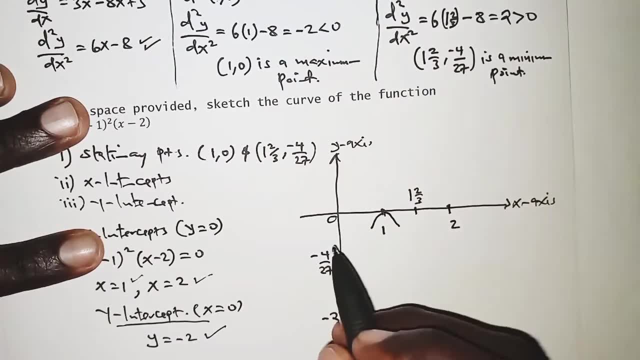 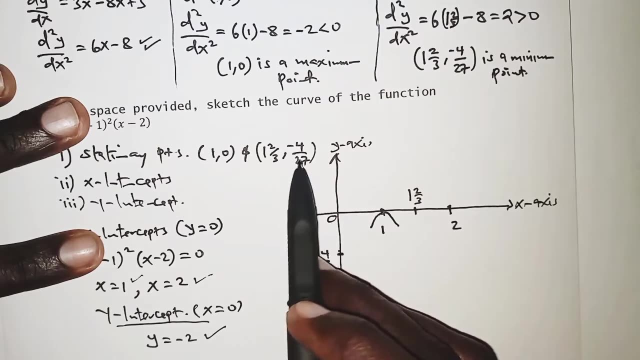 here is the origin. So if it's a maximum point, then the nature of the curve at that particular point is that for a maximum point. And then you also have 0.1 and 2 thirds negative, 4 over 27, as at this.